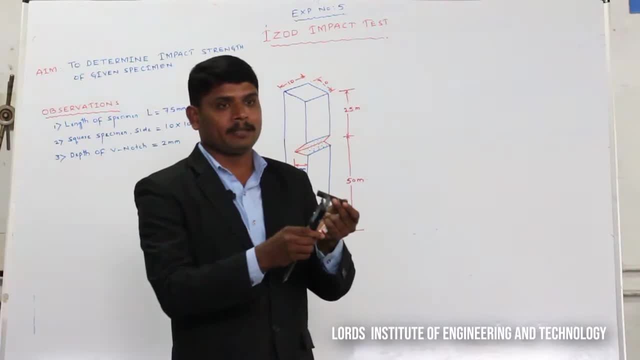 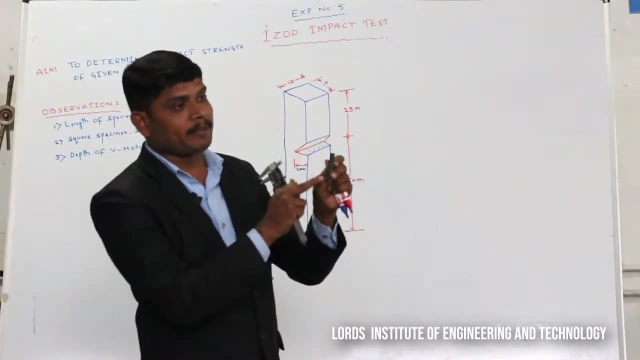 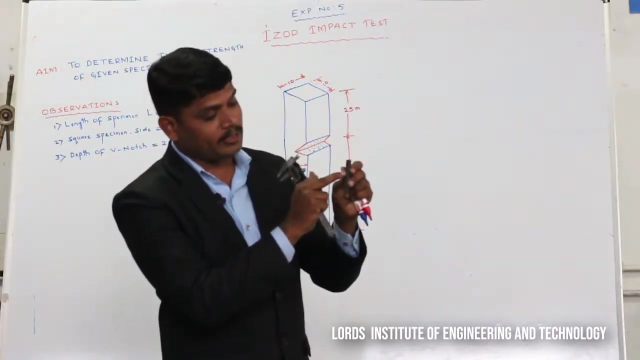 measuring the side of the specimen- square specimen- And now at a distance of 25 mm. total length of the specimen is 75 mm From any one end. I am taking top end, from the top side at a distance of 25 mm. I am. 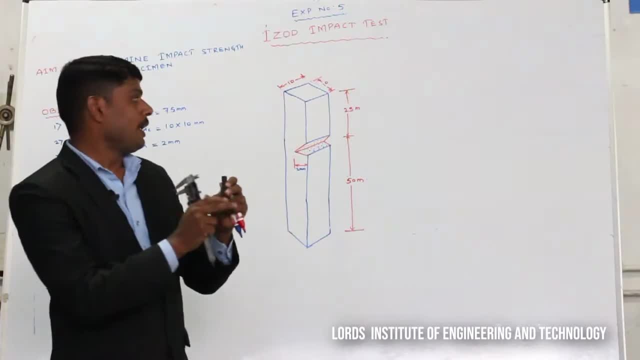 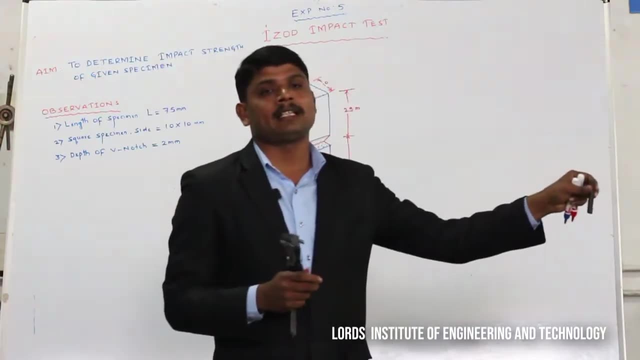 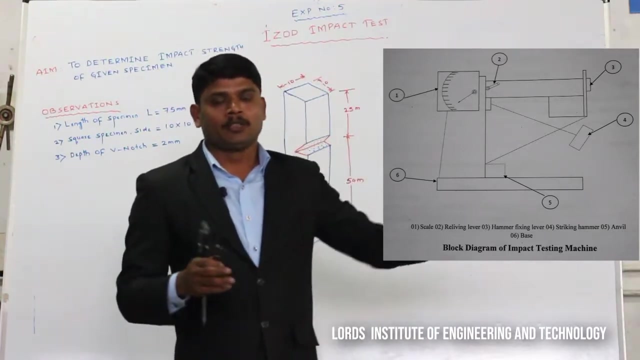 marking and I am growing a V groove whose depth is equal to 25 mm. So what I am doing? I will fix this specimen in a vice jar. Vice jars are placed in an anvil. Anvil is kept over the base of the machine. So we will perform the experiment now. So now so for performing. 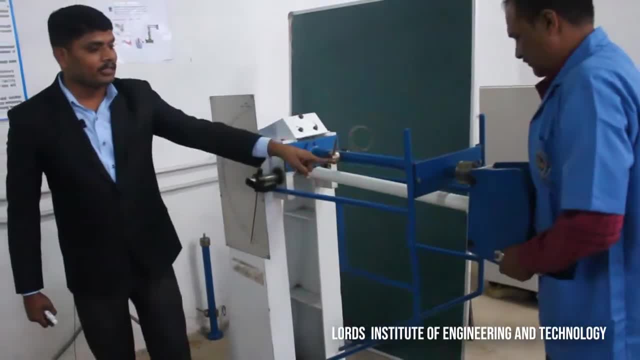 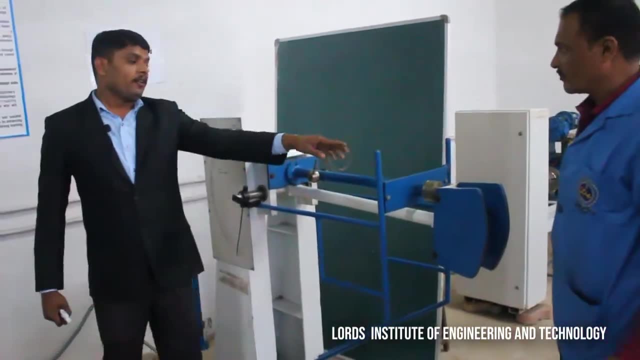 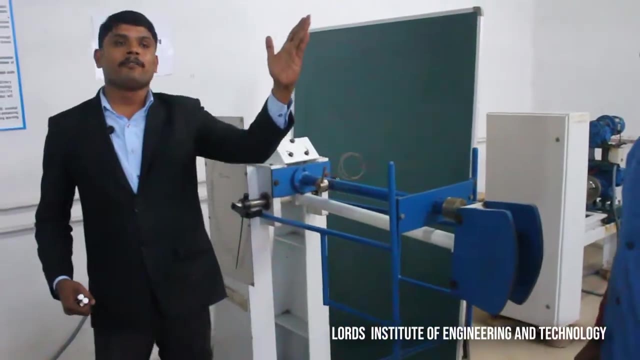 this IZOT test, we are lifting the striking hammer. This is what is striking hammer. We have lifted it up to a 90 degree and we have fixed it For releasing this. we have a one lever. If you operate this lever, what happens? This striking hammer will strike. 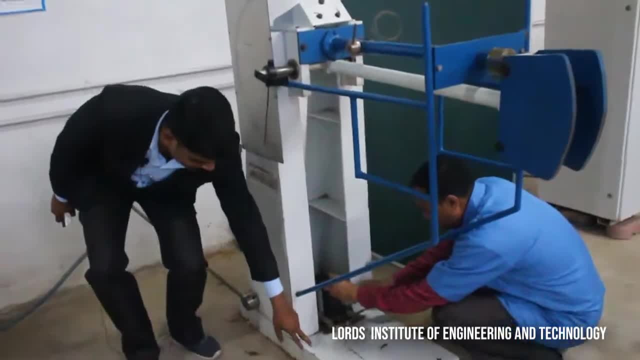 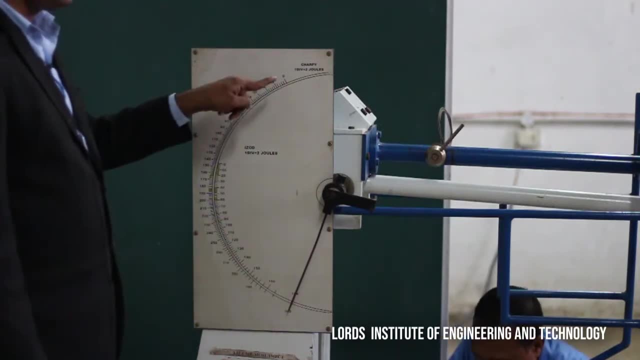 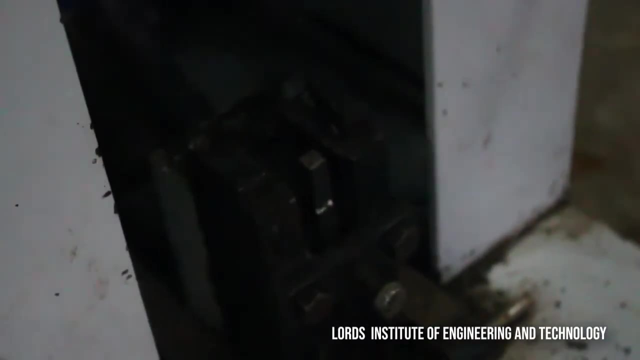 the specimen. So this is the base of the specimen, This is the arms and this is the scales where the reading is to be taken. So we have the two scales: One is the scale for IZOT test and one scale for Charpy test. 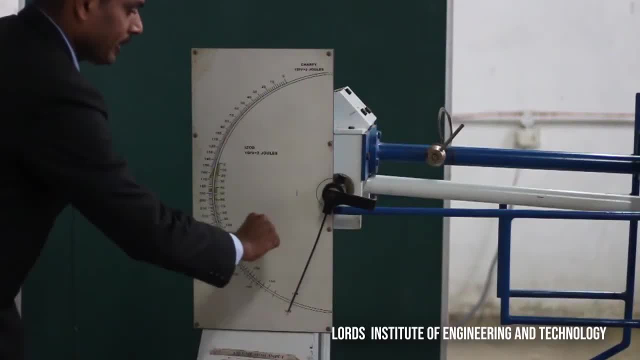 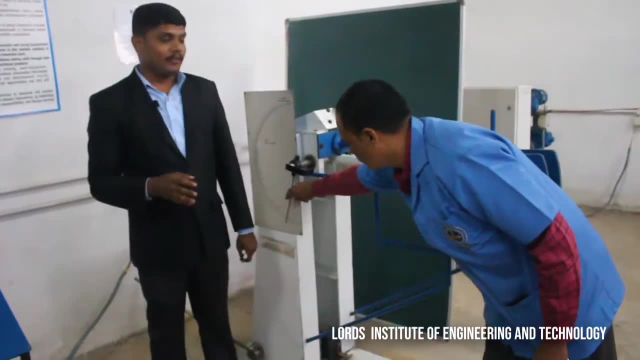 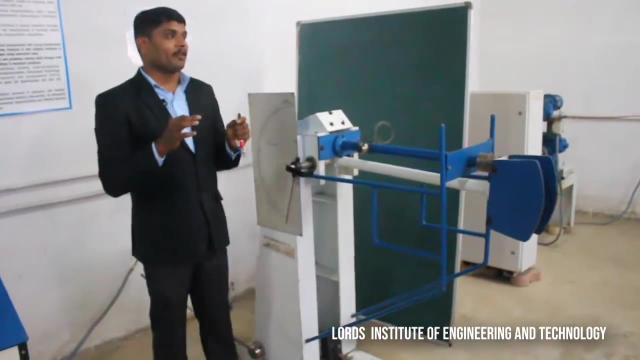 Inside the scale is for IZOT test. Here in this test we are measuring what is the energy absorbed before failure. We are performing the impact test when the striker strikes this specimen. So we have to find- we are seeing that- what is the energy absorbed before failure? 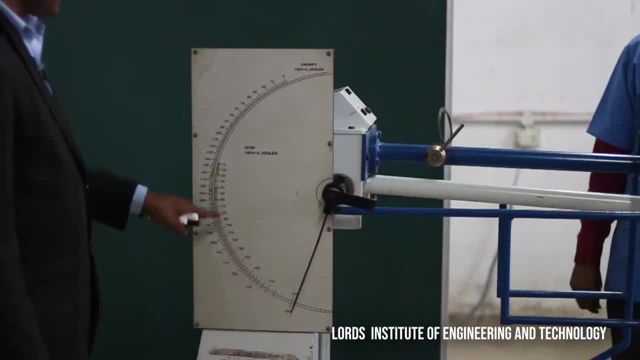 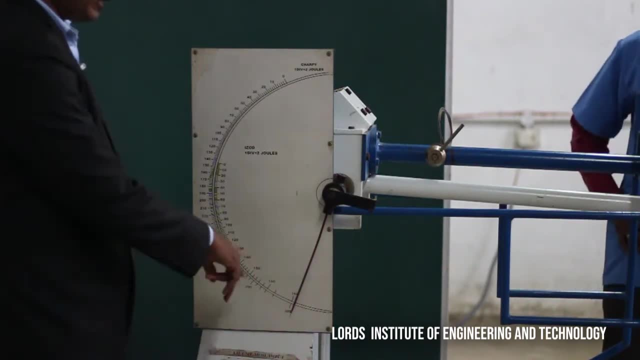 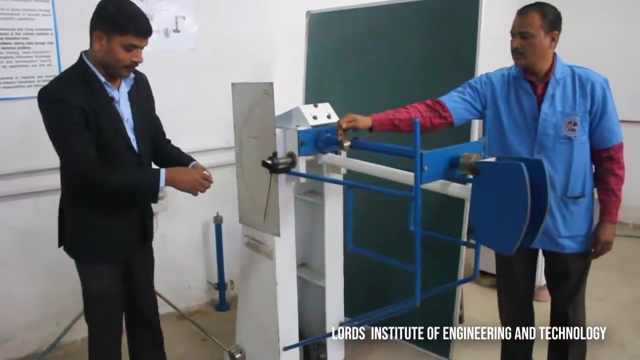 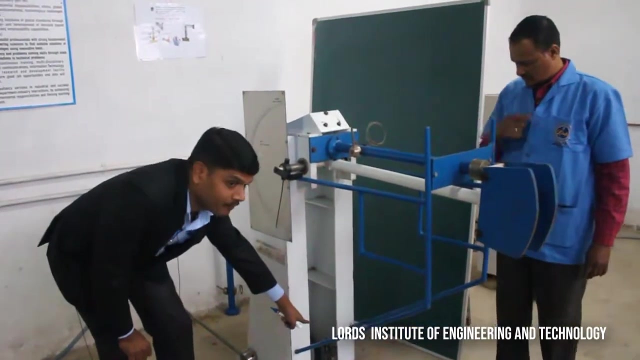 for the given specimen. Same energy can be calculated in this and it can be shown here in this readings. Okay, so now we will do one thing: We will release the lever. Okay, So one thing we can observe. One thing we can observe: We have placed a specimen, We 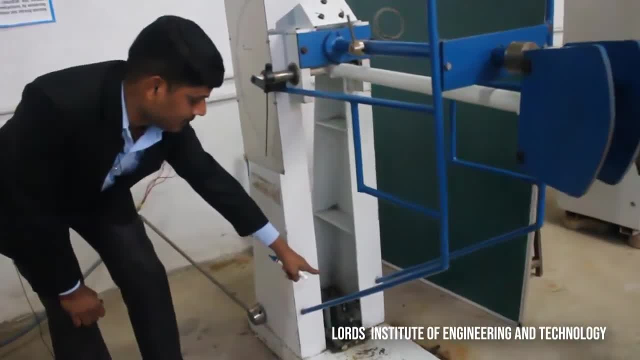 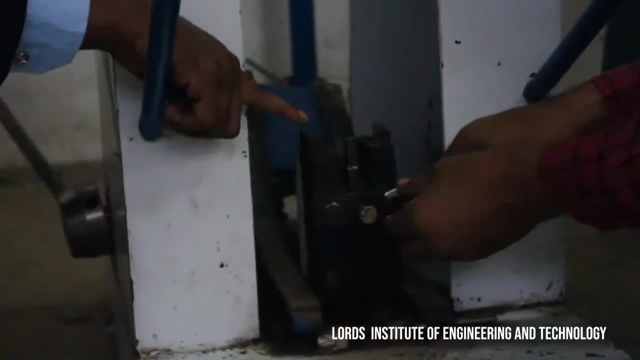 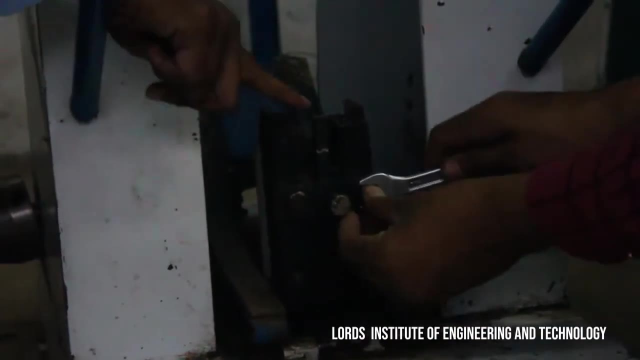 have placed a specimen in a jack vice And the jack vice is placed in an anvil And the anvil is kept in a. this is one specimen we kept here. We have placed in such a way that this notch is exactly coinciding with the striking part When we are releasing the. 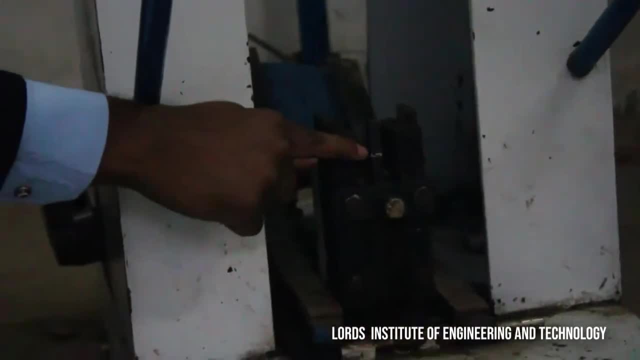 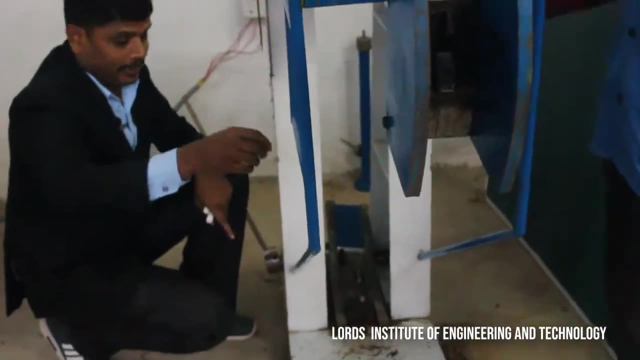 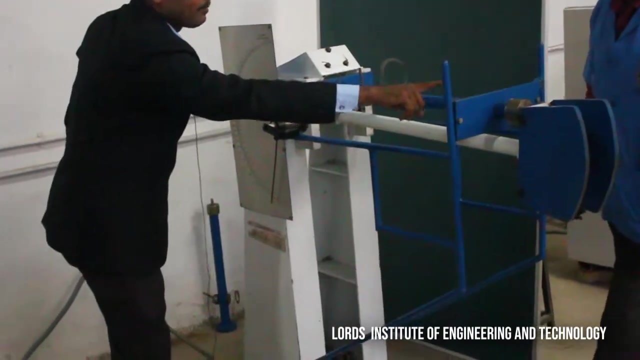 striking hammer. what happens? The striking part is exactly striking this particular point and it causes the break up of the specimen. Okay, So now I will what I will do: I will release the lever. After releasing the lever, this striking hammer strikes the specimen. 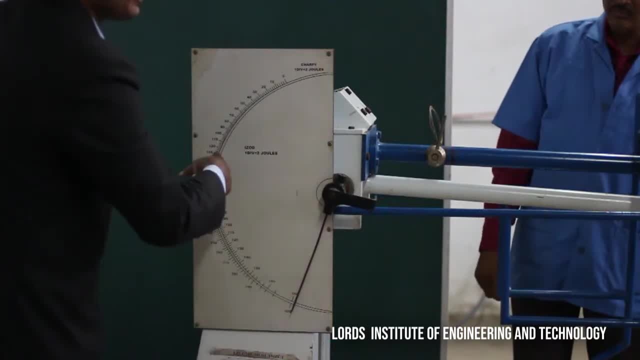 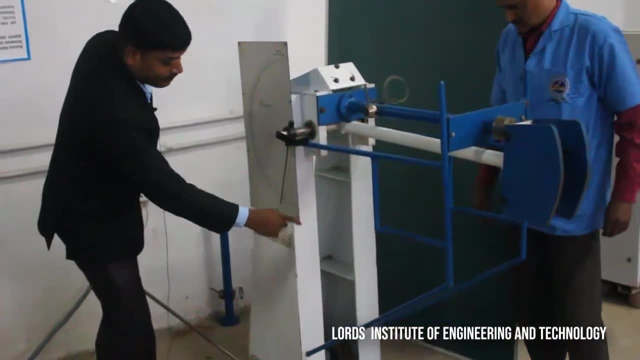 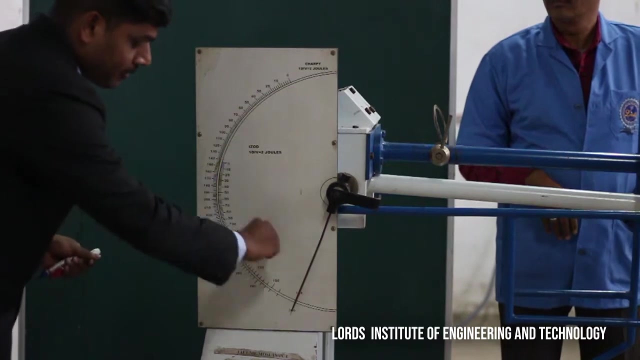 and now this pointer will move over the different graduations. It shows that what is the energy absorbed by that particular, this specimen, before failure? The pointer is on a 164.. We are seeing this inner scale, We are seeing the inner scale which is in terms of joule. 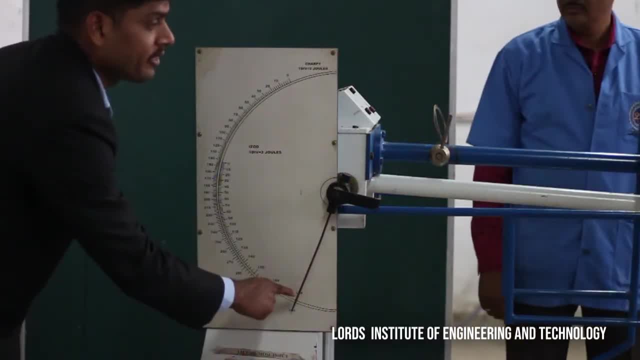 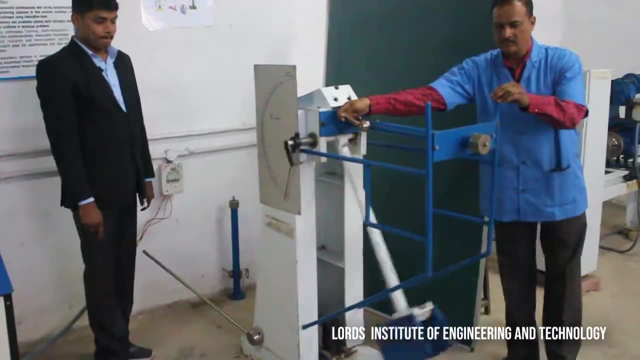 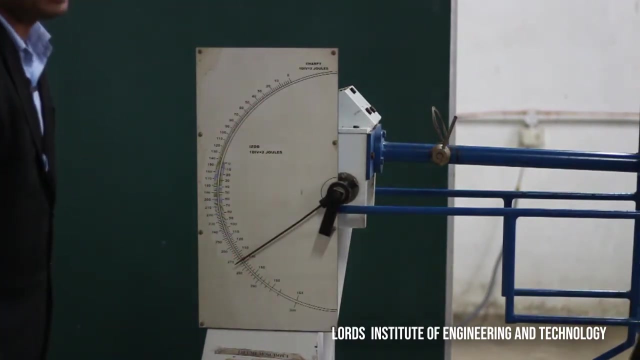 which is in terms of joule. So now initial reading is 164. before releasing the lever. Now we will release the lever. Yeah, So after releasing, we are observing that the pointer is on 140.. So we can say the energy absorbed by this specimen before striking it is 150 joules. 150,, sorry, 140. 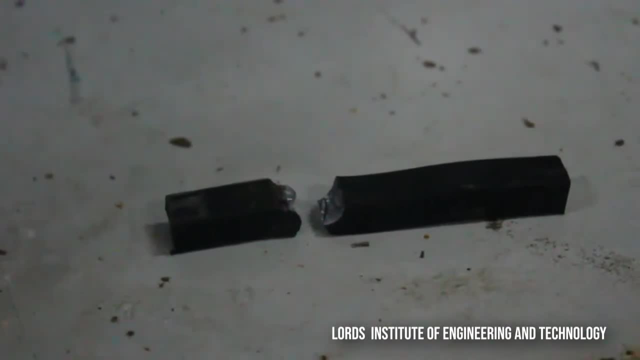 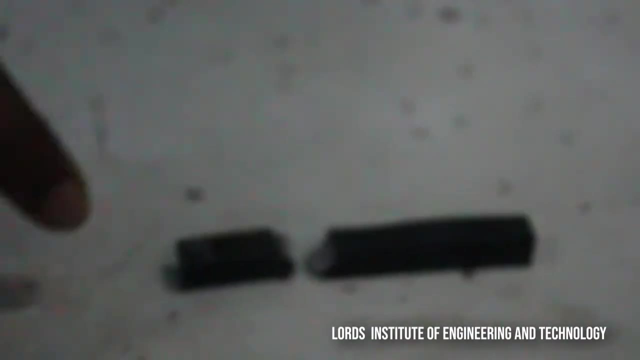 joules. Okay, So this is a specimen after striking the hammer. After when the striker hammer strikes, the specimen specimen is divided into two pieces. Okay, Okay, Hi there. This is Mohd M Bahutin, Assistant Professor, Mechanical Engineering Department. 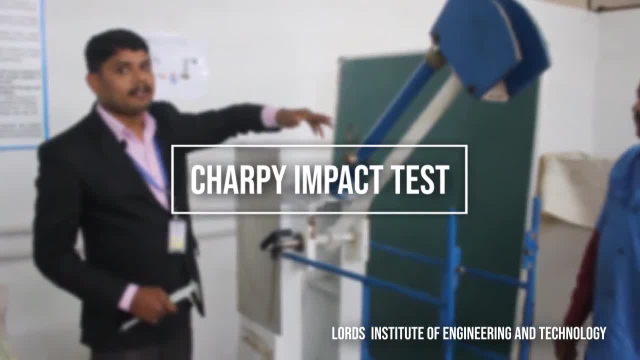 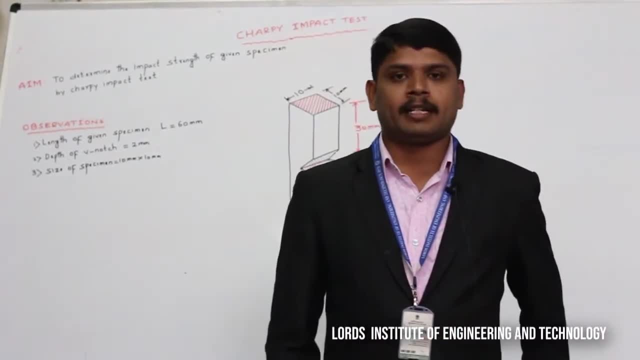 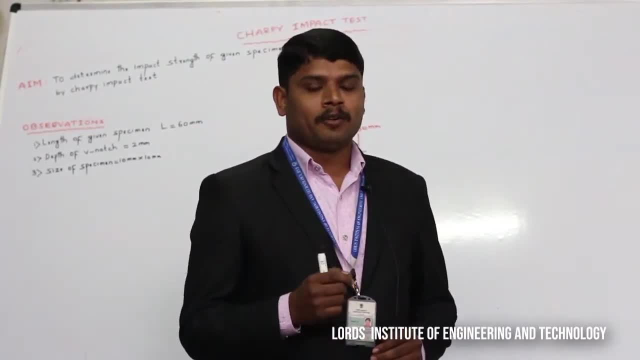 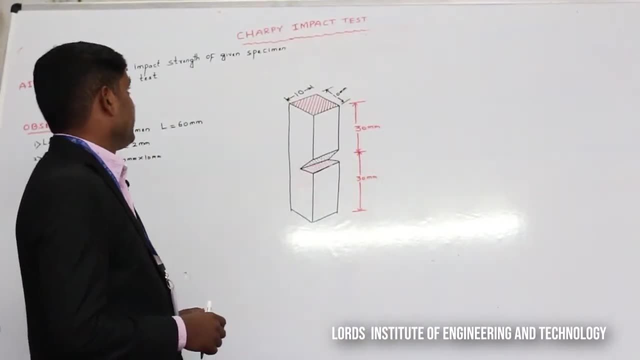 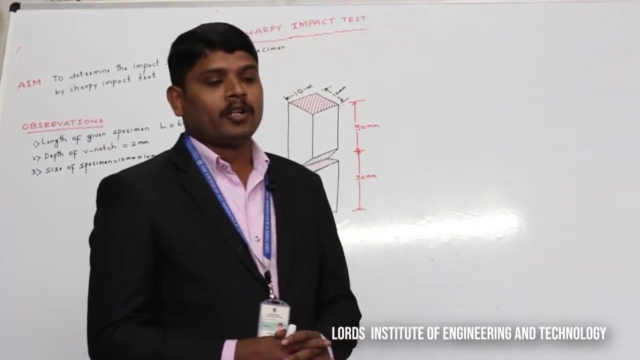 So the means of this tests is an enermical, interesting experiment. Now, in the sense of measurement, we are going to perform an impact Sharpe test. So the Zweاث Даmama experiment is to determine the impact distance of the given specimen. 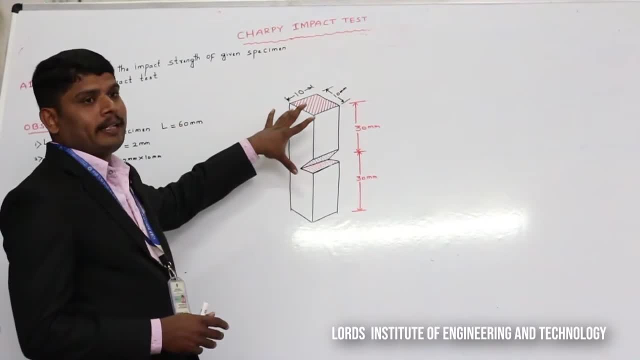 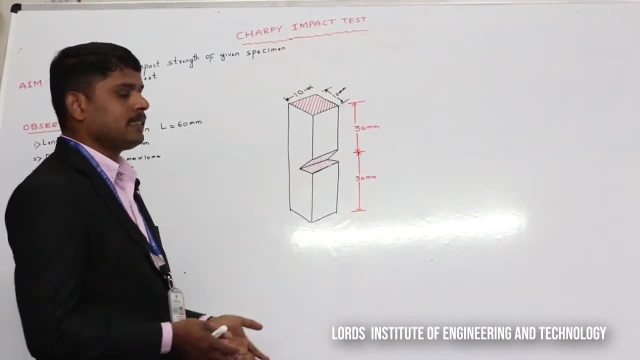 by using a Sharpe test. So we are going to perform the experiment. We have one about this specific thing. Okay, Okay, choose any material. it may be iron steel, it may be stainless steel, it may be any material. 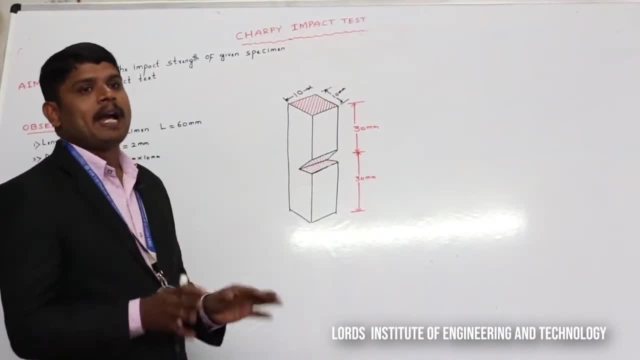 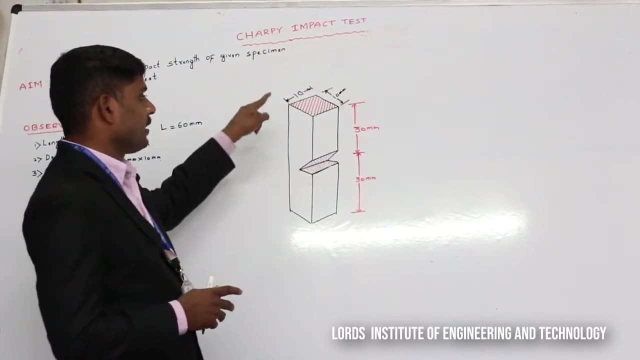 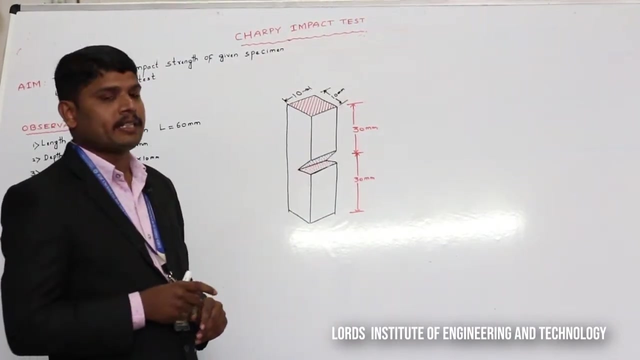 Our main aim is to find out the impact distance, that is, the toughness of the given specimen. So the standard sizes are: the total length of the given specimen is equal to 60 mm And this is square in shape. each side of this specimen is equal to 10 mm. 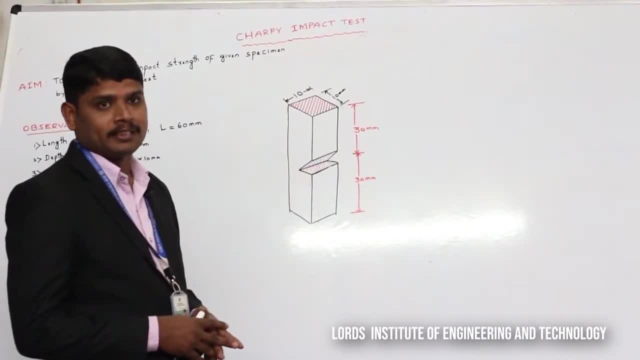 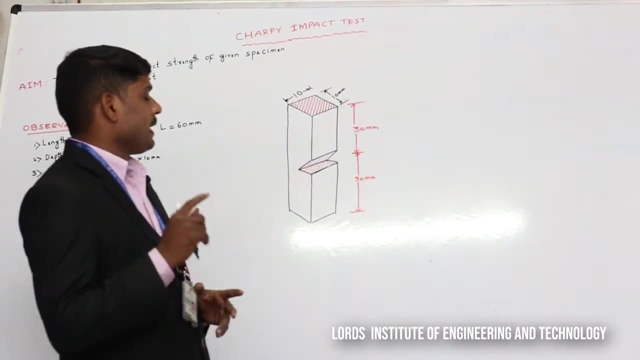 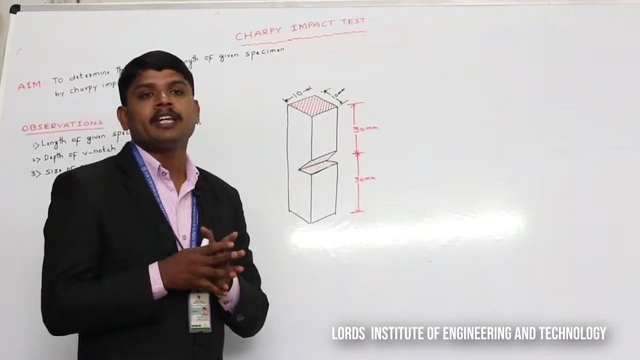 So 10 mm, 10 mm. this is square in size and the total length of the given specimen is 60 mm. Now, at a distance of 30 mm, either from the top end or either from the bottom end, we are making a V notch, V groove. we are making whose depth is equal to 2 mm. 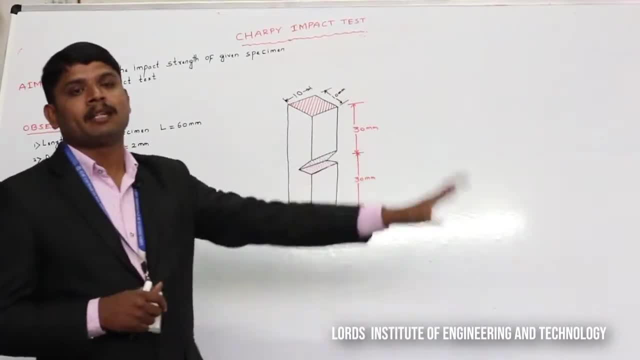 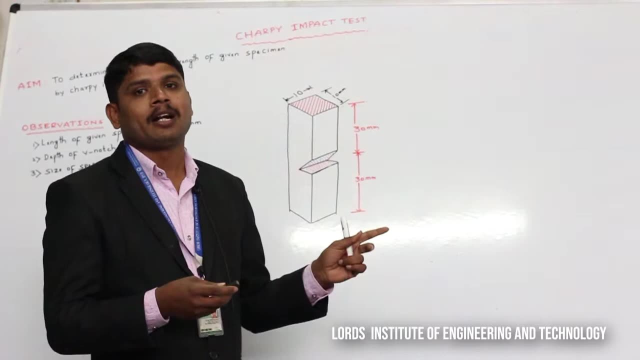 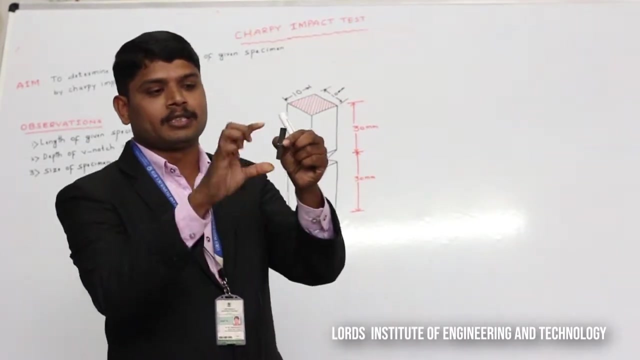 So what we are doing? we are placing this specimen in a vice and vice vice is kept in an anvil. And now what we are doing? by using a striker. the striker strikes the given specimen. So this is a specimen whose length is 60 mm and it is square in size, shape. 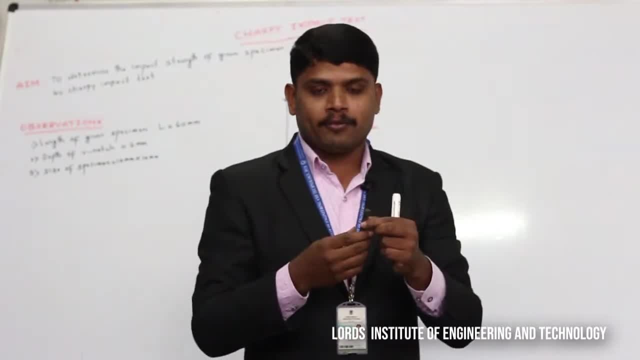 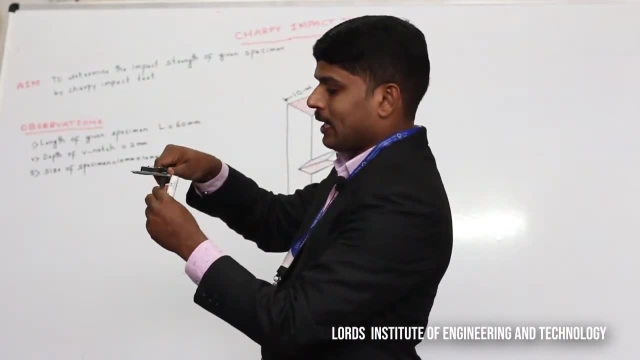 each side is equal to 10 mm. By using a vernier caliper, we are finding the dimensions, we are measuring, So each side is equal to 10 mm. 10 mm, Same thing we are. we will note down here. 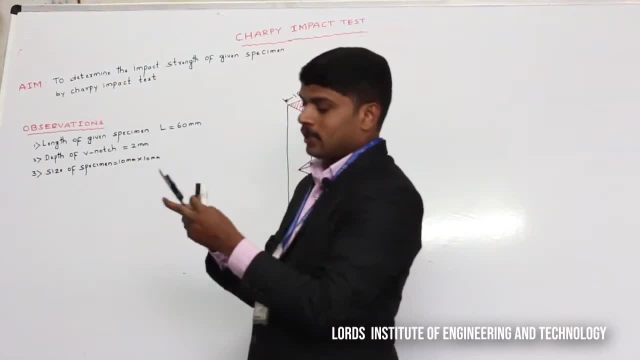 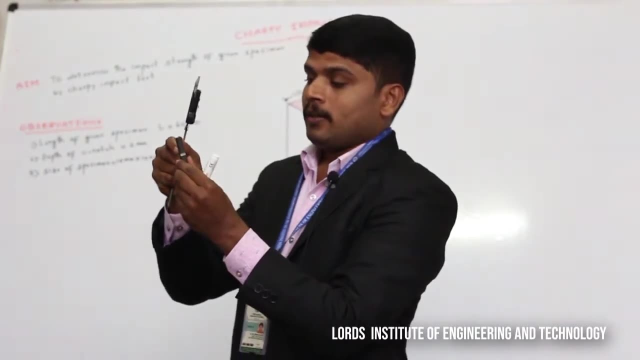 Each side is equal to 10 into 10.. Now we are making a groove- V groove- whose depth is equal to 2 mm. Now the total length of the given specimen we can find out by using a vernier caliper. 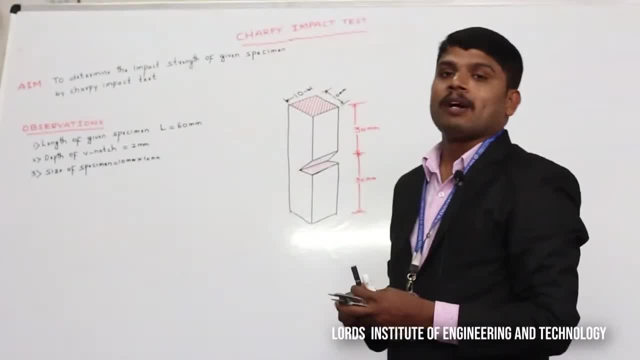 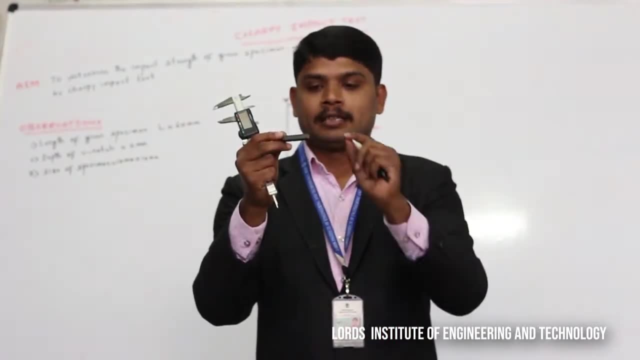 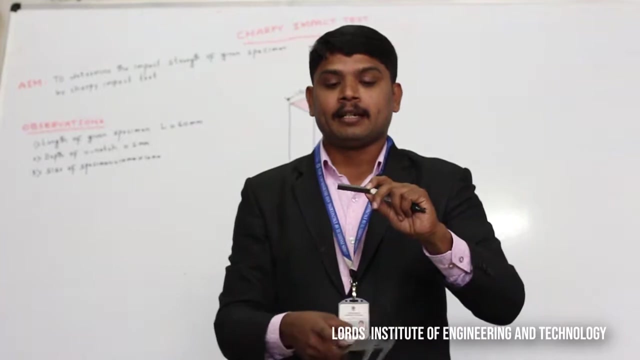 or by using steel root. So now what we will do? we will place this specimen in a horizontal direction. in a sharped test, This specimen should place in a horizontal direction on a vice. We are placing in such a way that the striker will exactly strike the notch. 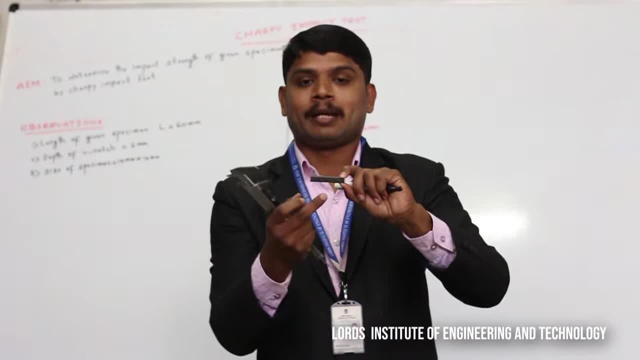 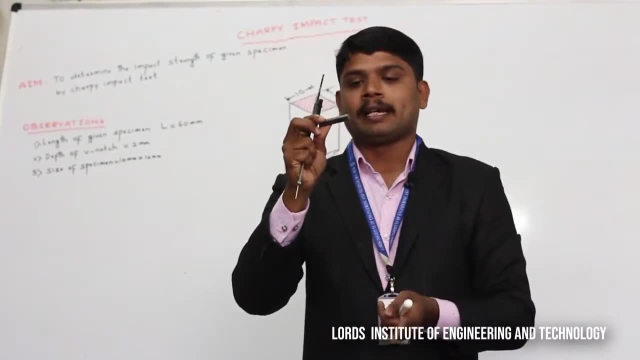 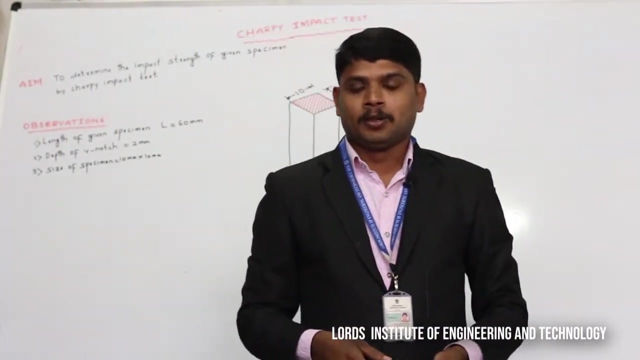 means the area of the notch. What happens because of striking? the specimen will break up into two pieces. So before breaking, before breaking, the energy absorbed by this given specimen can be found out by our device. So the main aim of our experiment is to find out the toughness. 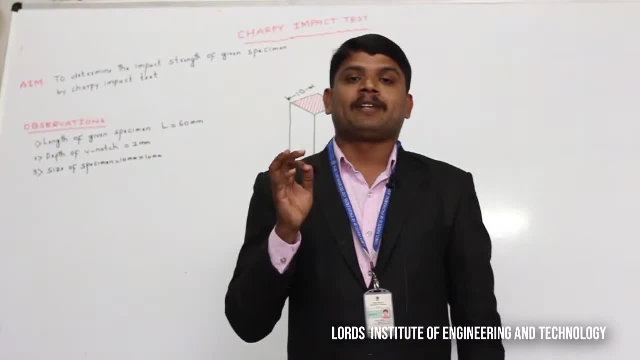 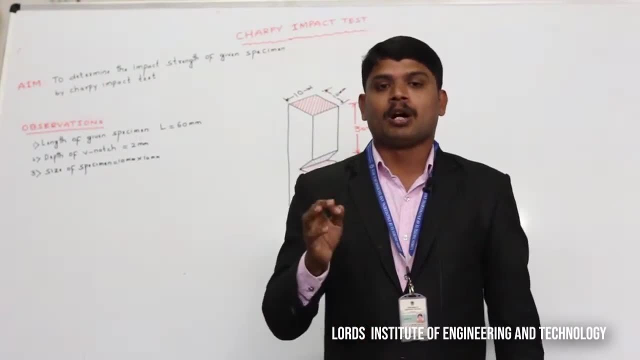 or we can say it is impact strength. The toughness is what? resistance to impact loading, resistance to failure against the impact loading. So now what we are doing? we are applying the impact load. So now we will see the experiment. Now this is a specimen. 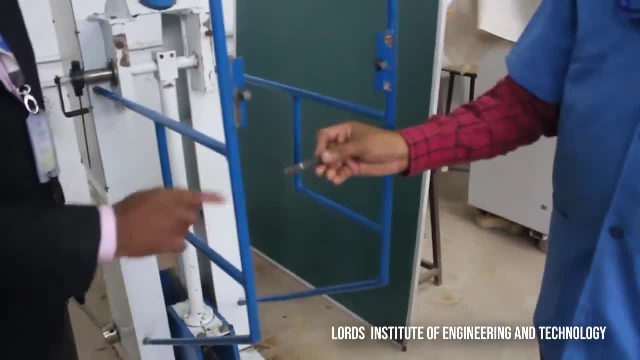 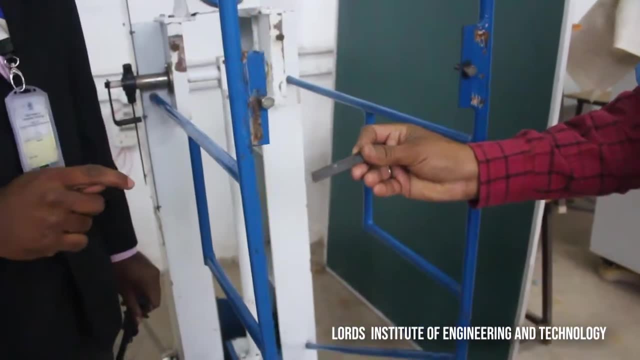 We know, this is a notch whose depth is equal to 2 mm. It is placed at a distance of 30 mm, So total length is 60 mm At a distance of 30 mm. we are making a V notch whose depth is equal to 2 mm. 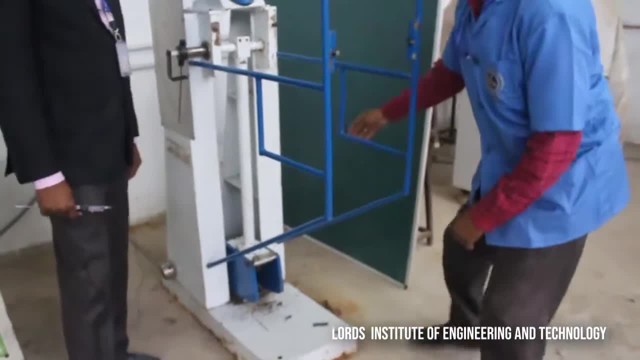 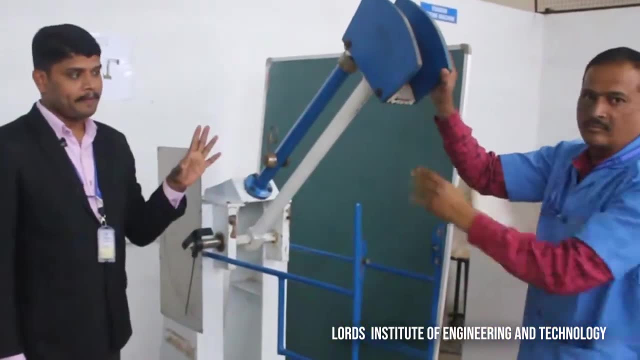 So now what we are doing? we are placing this specimen. So first of all, before placing, we are lifting this striker. We can say it is a striker and hammer, Okay, So this hammer is placed at an angle of 144 degree. 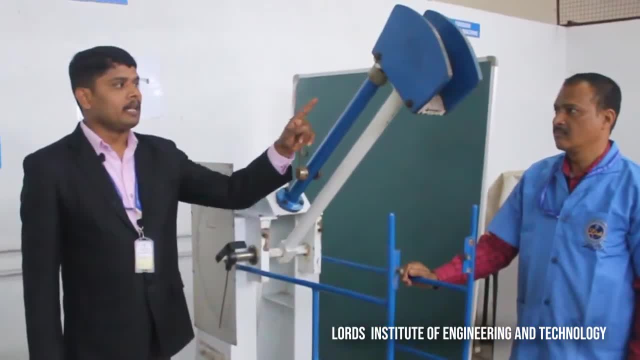 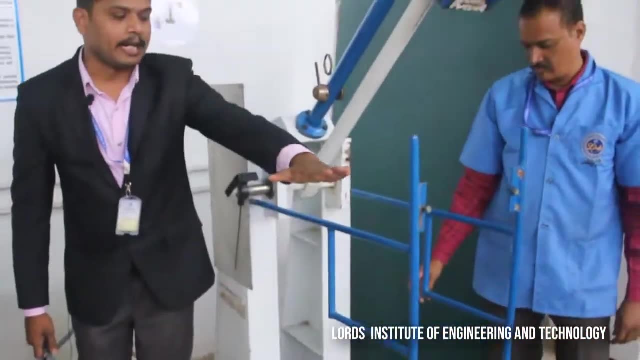 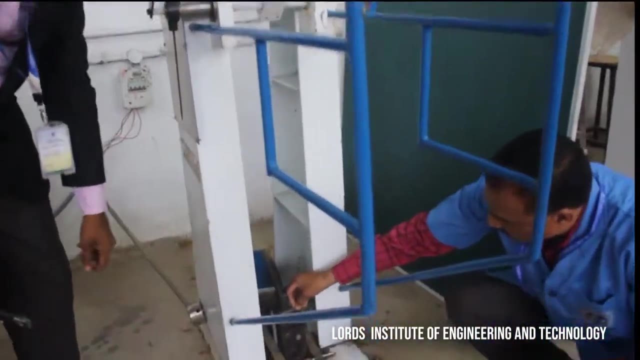 So for this, for this sharp test, the striker is placed at an angle of 144.. We can measure the angle from here. This is a 0, 90 degree And this angle is called 144.. Now what we will do? we will place this specimen in a vice. 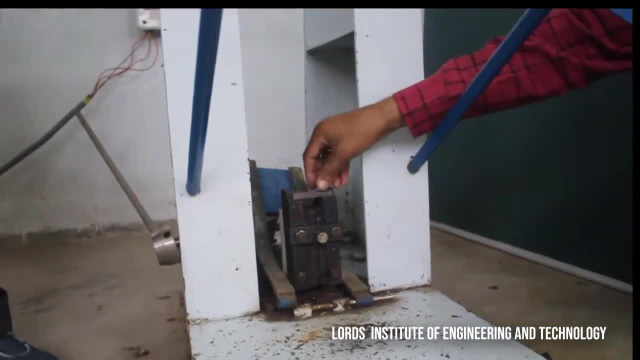 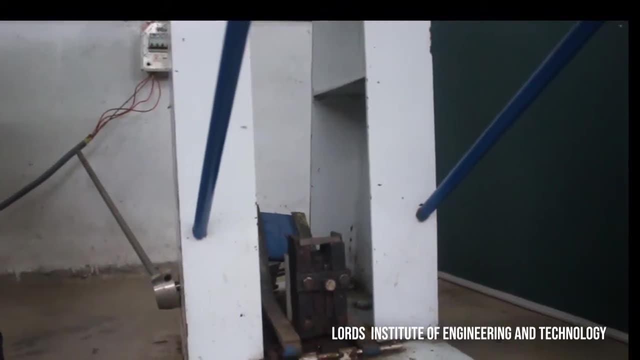 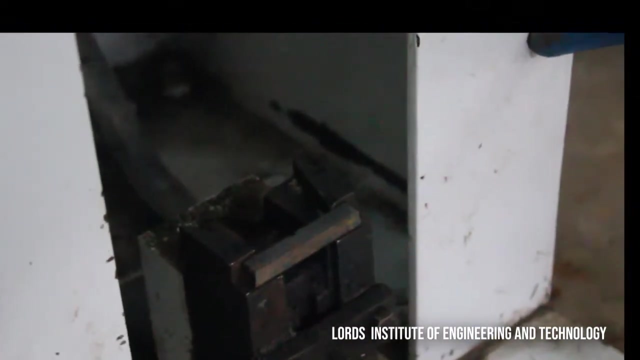 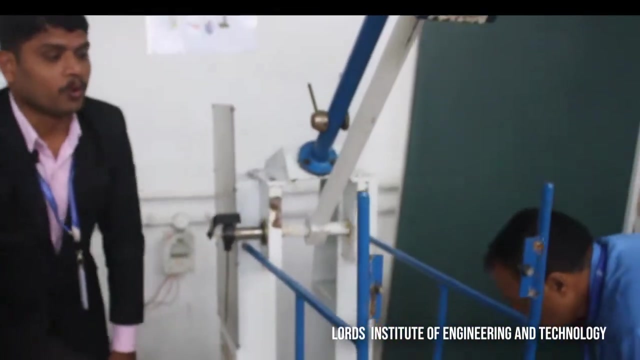 Okay, In a horizontal direction And notch is placed in a reverse, opposite direction to the hammer. Okay, So we are placing this notch in such a way that the notch is exactly coinciding with the striking part of the hammer. Now what? we will do. so for performing the hardness this impact test. 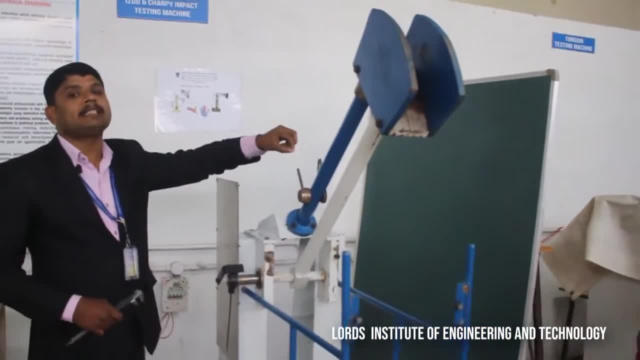 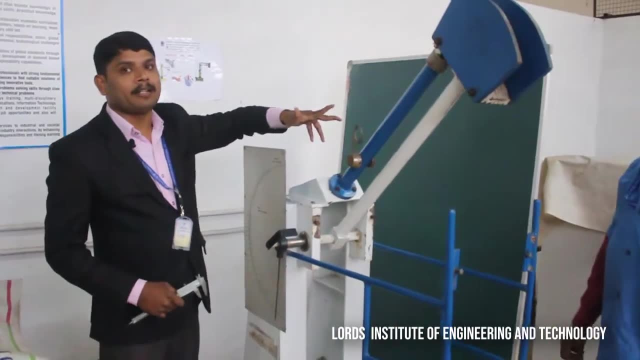 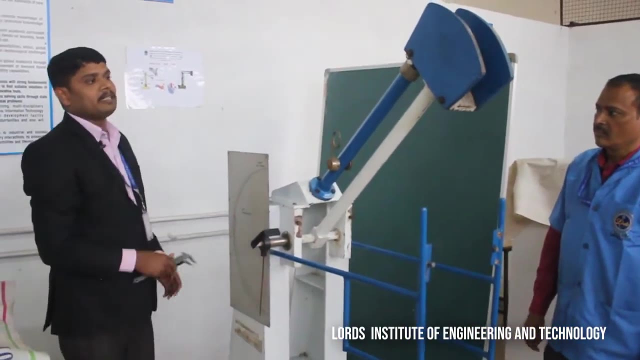 for performing this impact test. what we will do? we will release this hammer. We will release this hammer. We have one of the lever, Okay. So when we release the lever, what happens? This striker strikes the given specimen. So, before releasing this hammer, we will see that this pointer should be on a 300.. 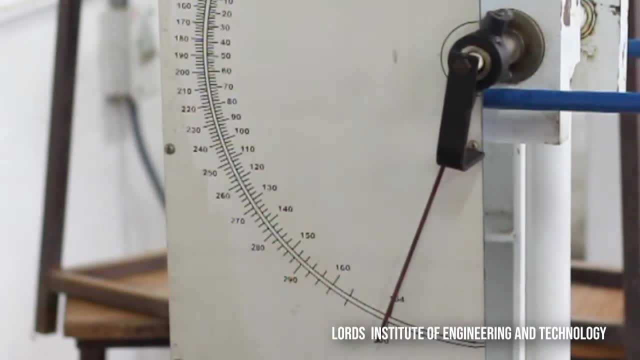 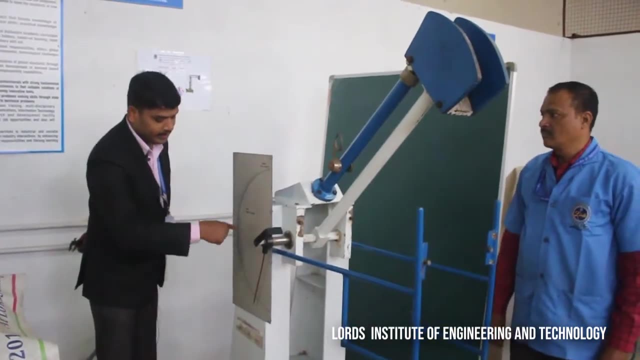 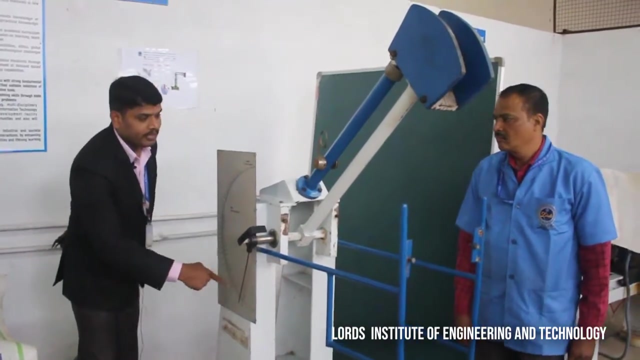 It should be on a 300.. So our experiment is sharp test. So there are the two scales: Outer scale is there and inner scale is there. So inner scale is inner graduations we are using for ISO test, And outer scale graduation we are using for sharp test.